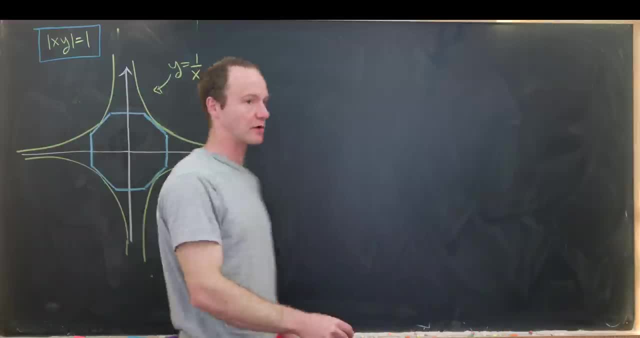 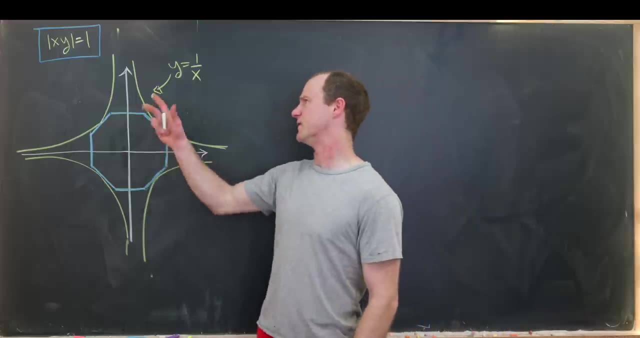 we'll just consider this portion of the curve, which is: y equals 1 over x. Then, furthermore, we've got this octagon, which is inscribed inside of this curve, And so it's a regular octagon. That means all of the sides are equal. 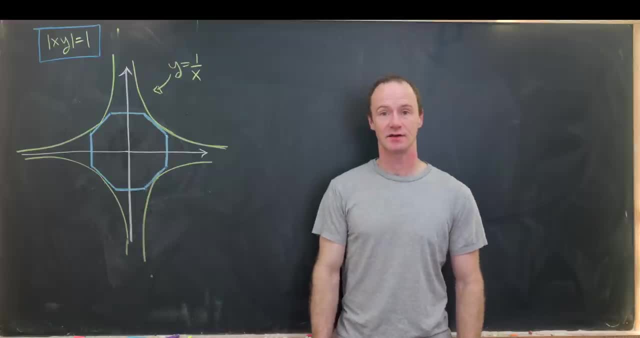 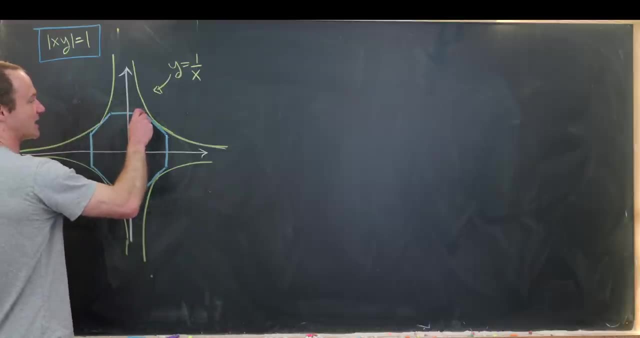 And then our goal is to find the area of this octagon. So, first off, what I'd like to do is notice that I'll be in good shape if I can find this coordinate right here and this coordinate right here, And that's because I can break this into the area of something that's happening in the first quadrant. 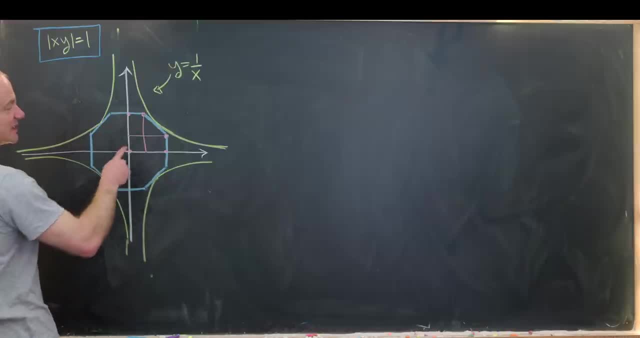 by kind of excising this into pieces And it's pretty easy to find the area of each of those pieces. But in order to find these two points right here, what I'll need to do is hone in on this point. where this leg of the octagon is tangent to the curve, y equals 1 over x. So let's figure that out. 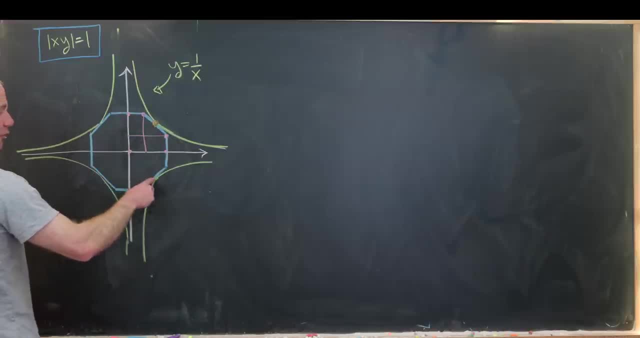 Now, first of all, by symmetry, we see the x coordinate and the y coordinate, for this point has to be the same, just by reflecting down across, and so on and so forth. So, since the x coordinate and the y coordinate have to be the same, and it's on the curve, y equals 1 over x. 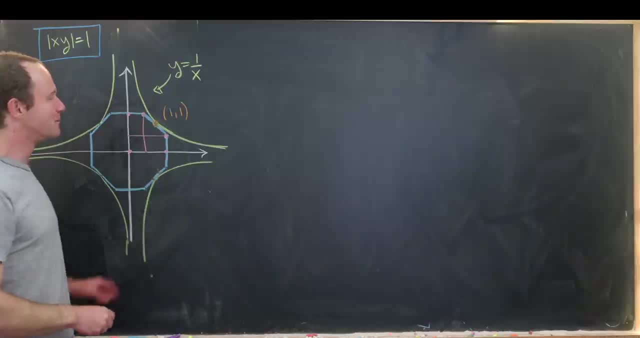 we know this coordinate right here is 1 comma 1.. That helps us out quite a bit to find the equation of this tangent line, The tangent line which is really just the linear extension of this leg of the octagon. Okay, so let's find the equation of this green tangent line I'm drawing: 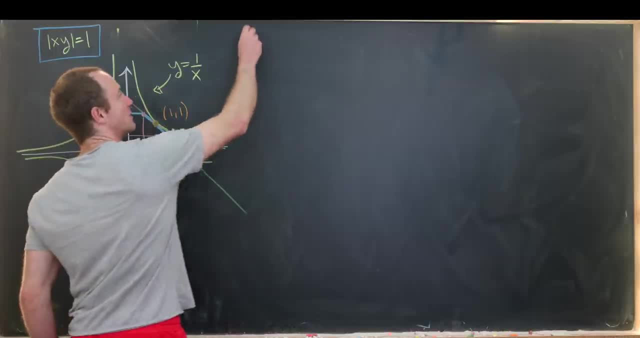 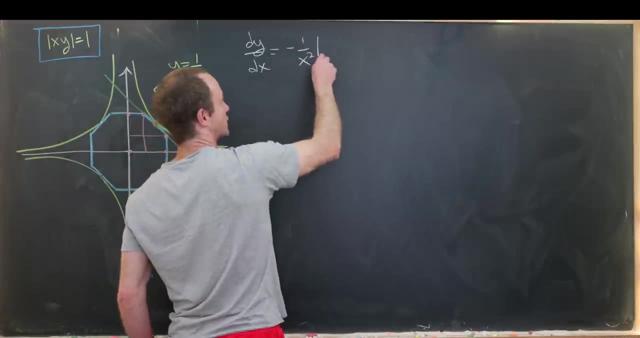 So we know a point on the line, which means we just need to know the slope. We can find the slope by finding the derivative with respect to x of 1 over x. That clearly gives us 1 over x squared. We plug in x equals 1 and we get a slope of. 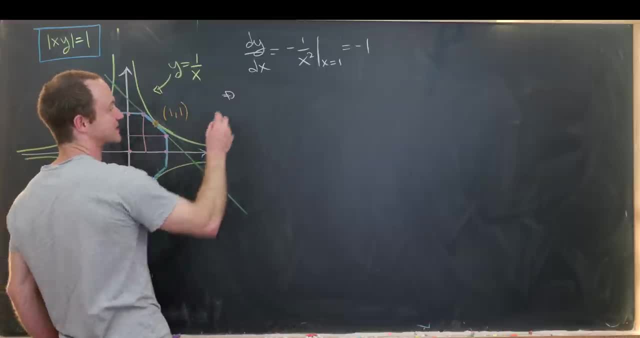 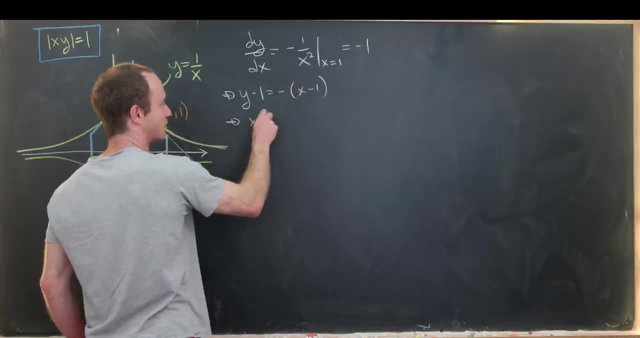 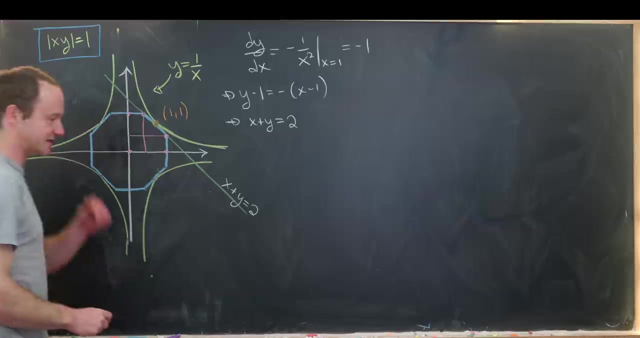 negative 1.. So that means by the point slope form we have an equation- y minus 1 equals negative x minus 1, which can be rewritten to x plus y equals 2, which is actually the way that we're going to think about it. That will be most useful for our purposes. 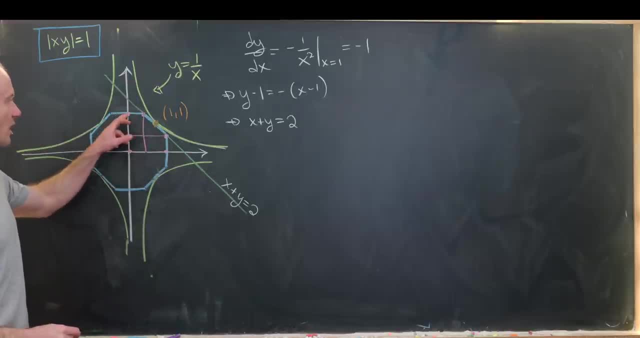 Next up. we need to close some conditions on these points right here in pink. So I'll give them names maybe. So let's say that this is coordinate a, this is coordinate b and then by symmetry up here on the y axis will be a and this will be b. That makes this point right here equal to a comma b and that 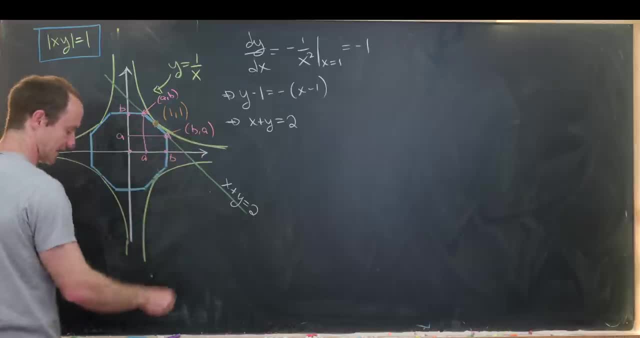 makes this point right here, equal to b comma a. Now, since this is a regular octagon, we need the distance between 8 and the generation to the length 2a to be exactly double the length of a, and that's because 2a is the. 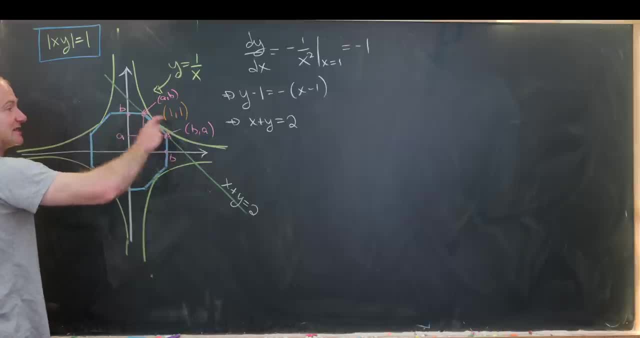 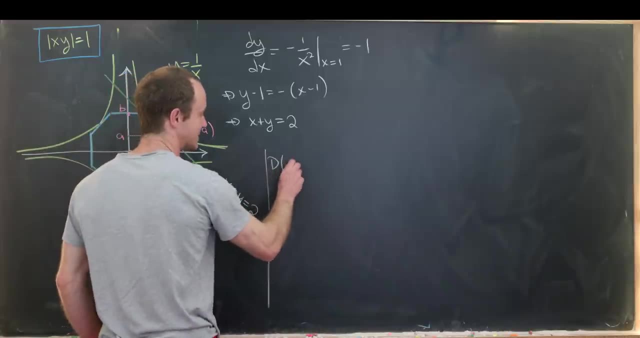 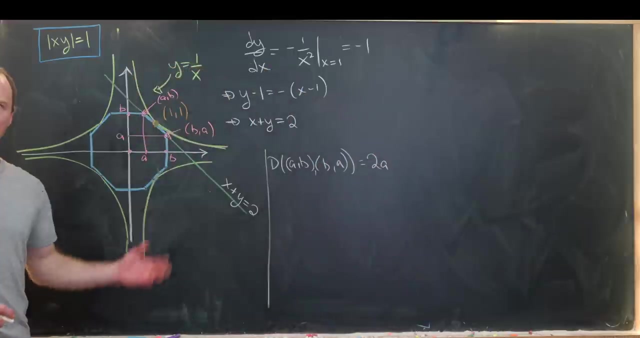 length of this side right here, and we want all of these sides to have the same length. Okay, so now let's impose that condition over here. So, like I said, we need the distance between point b to be equal to twice a. Now let's use the distance. 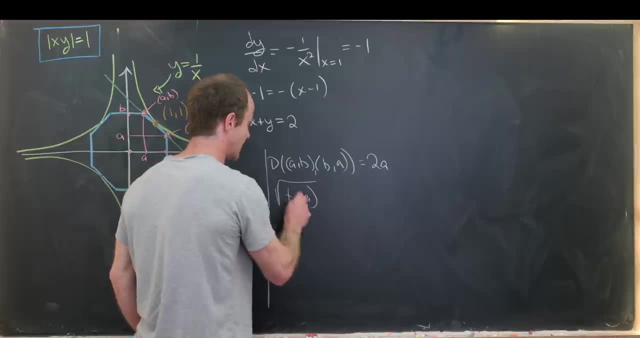 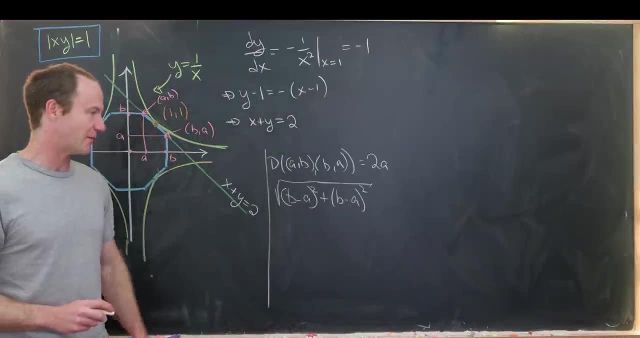 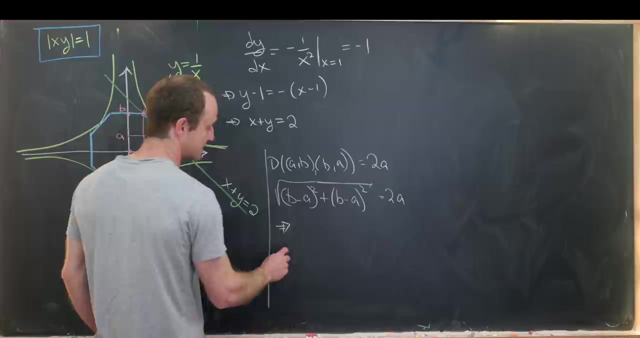 that gives us the square root of b minus a squared plus b minus a squared, where I've used the fact that since I'm squaring, that I can flip as needed, because now I have the same thing in there is equal to 2 times a. but now, putting that all together, we see that the square root of 2 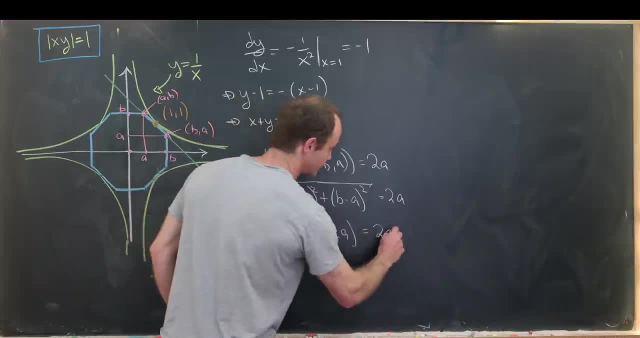 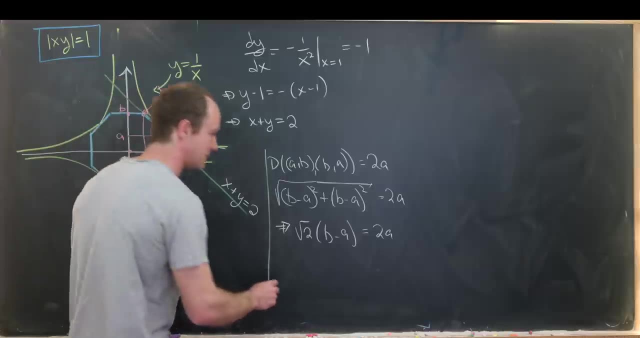 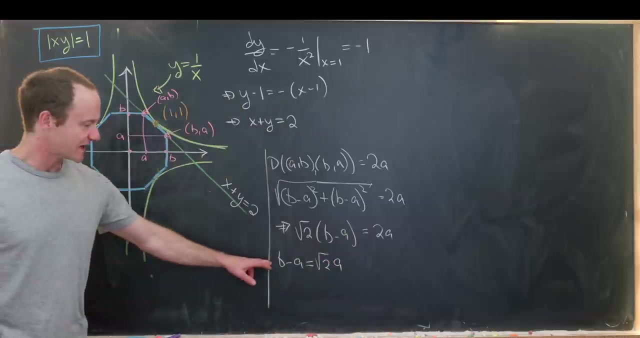 times b minus a is equal to 2 times a. that's because we get 2 times b minus a squared and then we take the square root of the whole thing. so that means we get b minus a equals 2 over root 2. but that's just root 2 a. but there's actually another equation that's satisfied up by a and b. 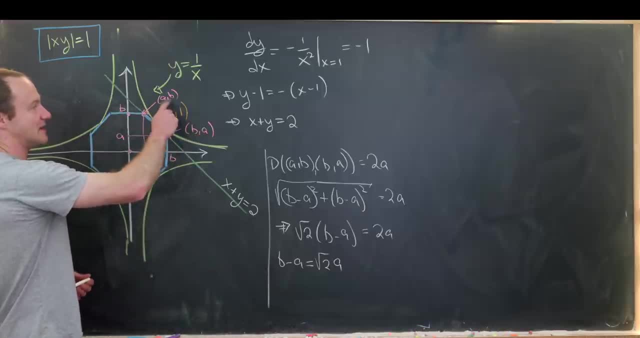 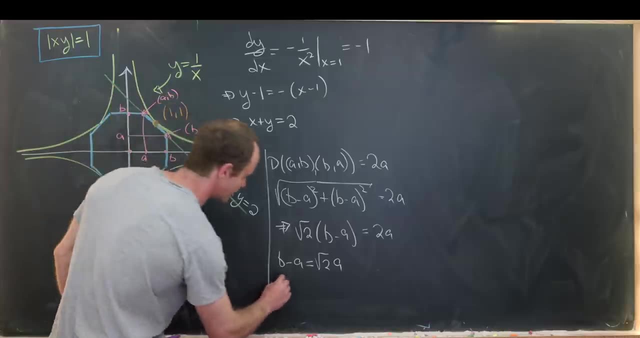 also, and that's because this b comma a and this a comma b are also points along this tangent line that satisfy this equation. so that means we also know that b plus a equals 2.. Okay, so now we're in a pretty good spot, So let's take 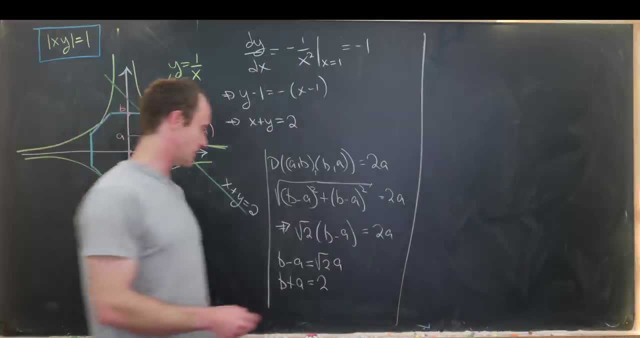 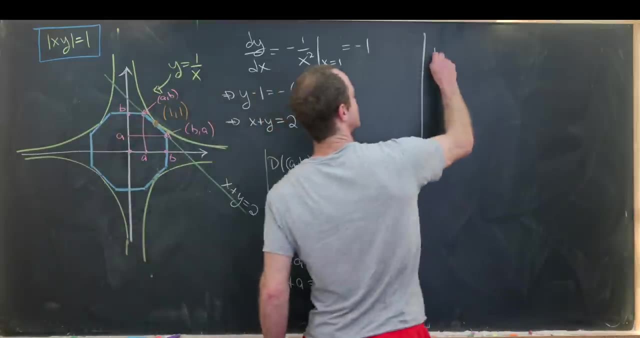 that and find the longiasочка, those two equations, and see if we can solve for A and B. So maybe the easiest thing to do is to solve this first equation for B and then plug that into the second equation. So let's notice that B is equal to one. 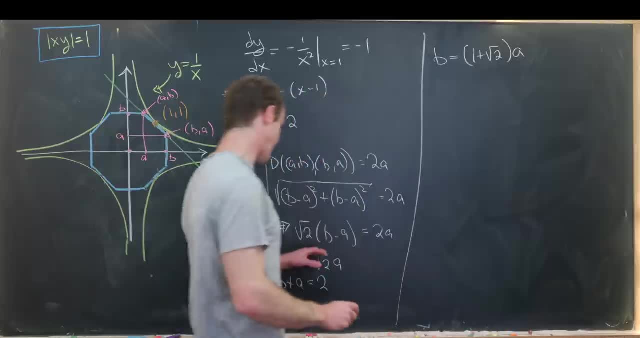 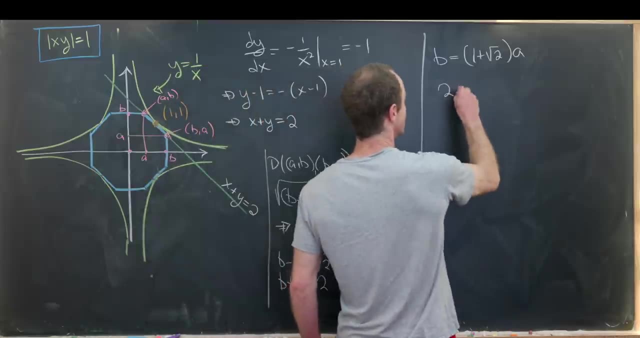 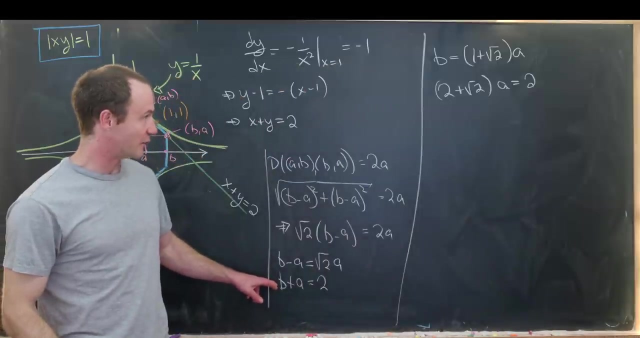 plus the square root of two times A. We get that after factoring things out, But now, plugging that into the second equation, we get two plus the square root of two times A equals two. So that came from the fact that we've got another A. 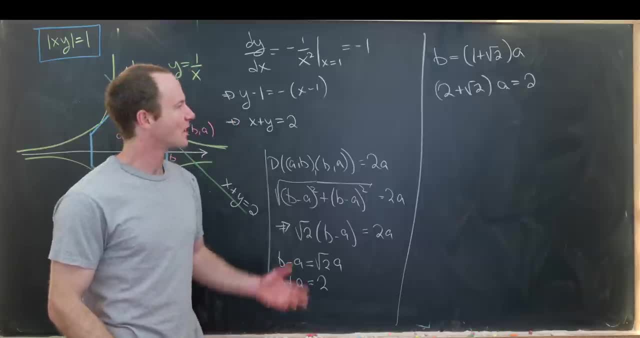 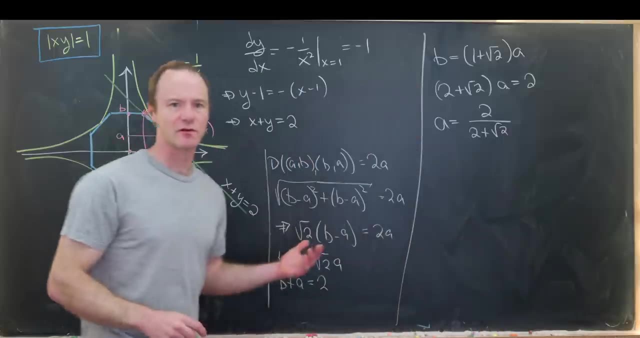 to add in. that turns this one into a two. Okay, but that tells us that A is equal to two over two plus the square root of two. And since we've got several more calculations coming down the line, I'm gonna go ahead and rationalize the denominator here. 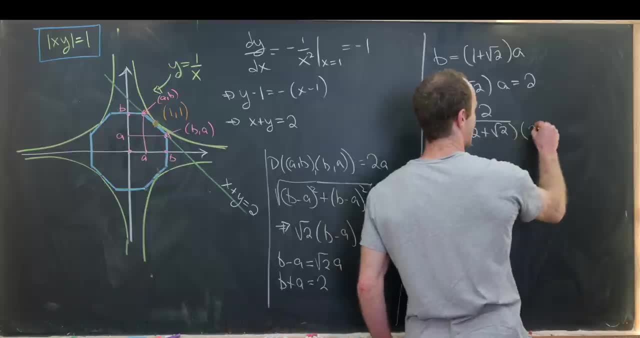 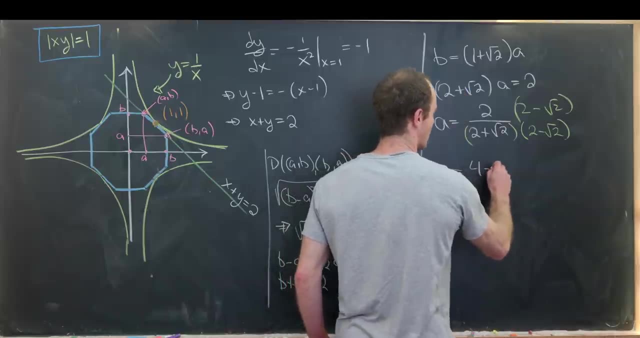 So in order to do that, I'll multiply the numerator and the denominator by two minus root two. So there we've got that. So that leaves me with four minus two root two in the numerator, And then, downstairs, I'll be left with two times two. 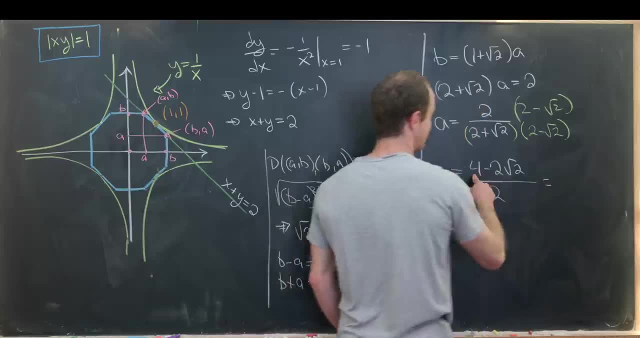 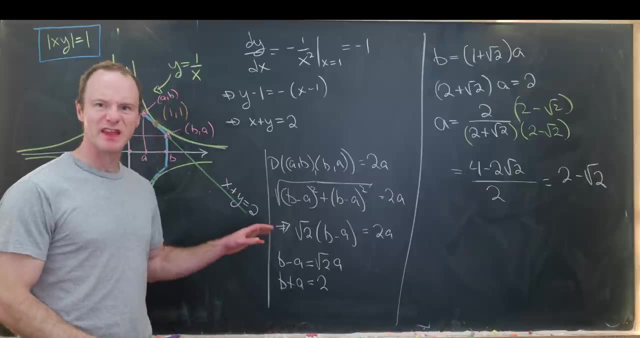 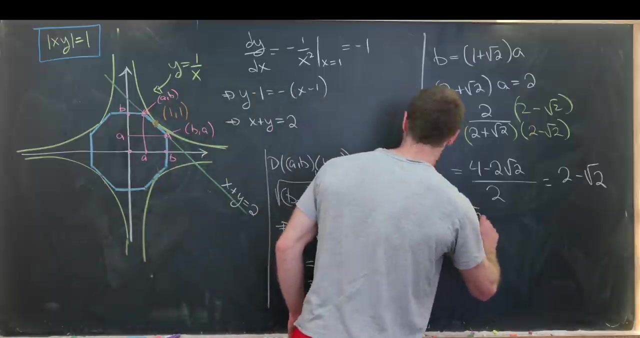 which is four minus two, so that's two, And then, simplifying, I get two minus the square root of two for our value of A. Now maybe the easiest place to plug that value of A, to find B is right here, and we'll see that B is equal to the square root of two. 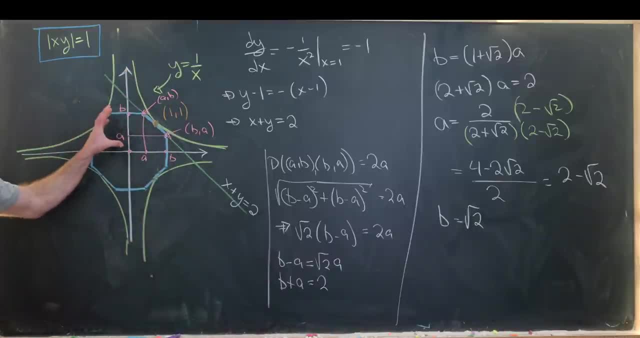 Okay, so we could fill in those values of A and B right here, but I think that would make that a little bit too messy. So what I'll do is erase all of this and we'll blow up what's happening in the first quadrant. 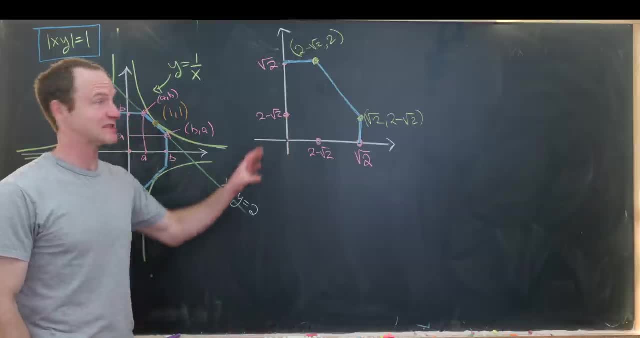 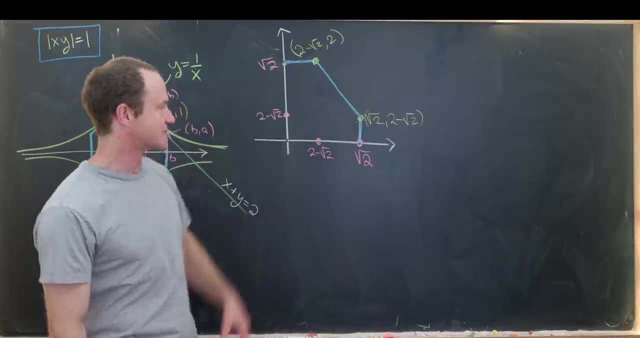 Okay, so here's an expansion of what we solved for on the last board, but just in the first quadrant. So our goal area, which is the area of this octagon, will indeed be four times the area of this picture that we have right here. 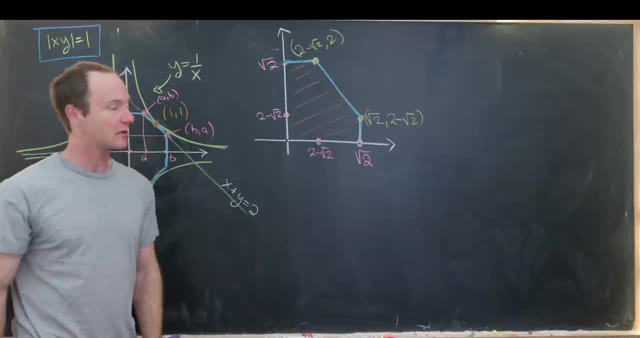 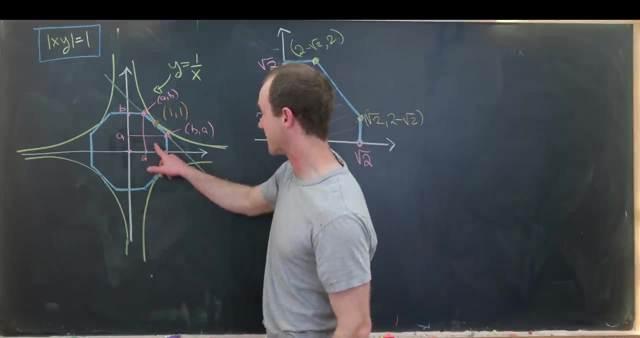 So let's see this. brown is the area that we'll calculate now. Now we could do this a number of different ways. We could cut this over here, like we've done, into two rectangles, a square, and then this triangle up here. 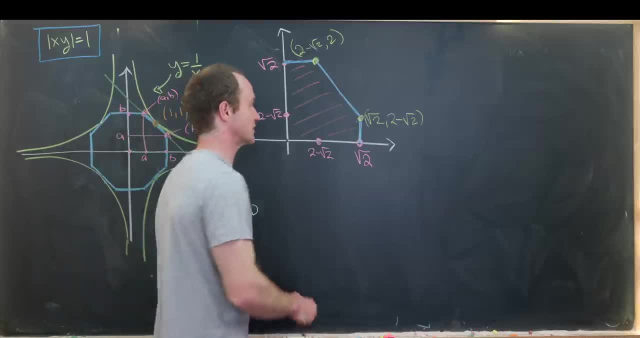 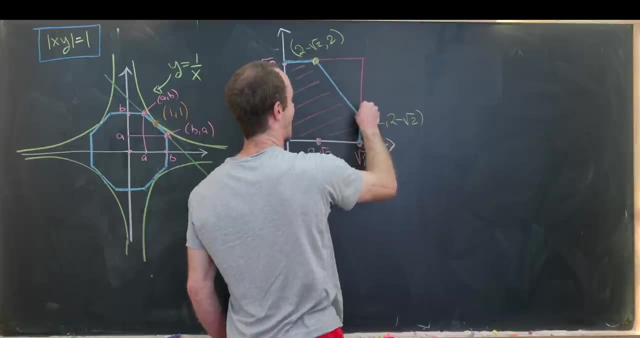 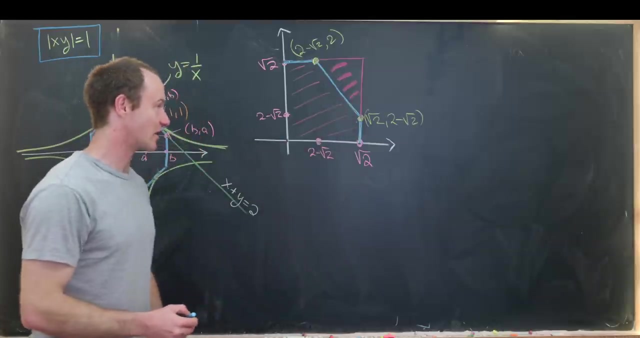 But instead of doing that, let's extend this picture a little bit by completing this into a square, And then notice that our area that we're interested in will be equal to the area of the square minus the area of the triangle. Furthermore, it's easy to calculate the area. 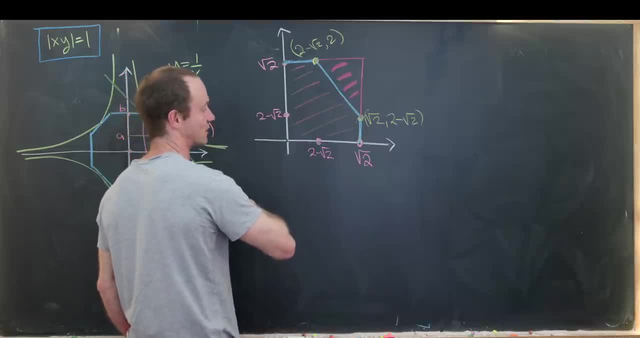 of this triangle because first of all it's an isosceles triangle. That's by symmetry, but also just by checking that the length right here is equal to- let's see- the square root of two minus two minus the square root of two. 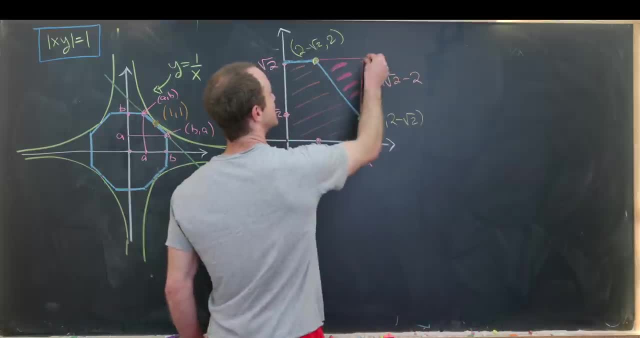 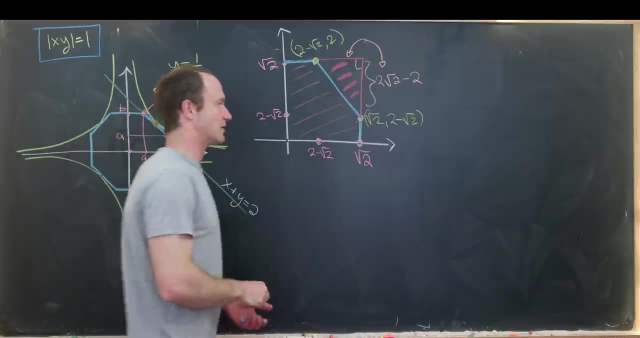 So that gives us two root two minus two, And that's gonna be the same thing as this length right here. Furthermore, it's a right triangle, So that means we can just multiply those and divide by two, So in the end we'll get the area. 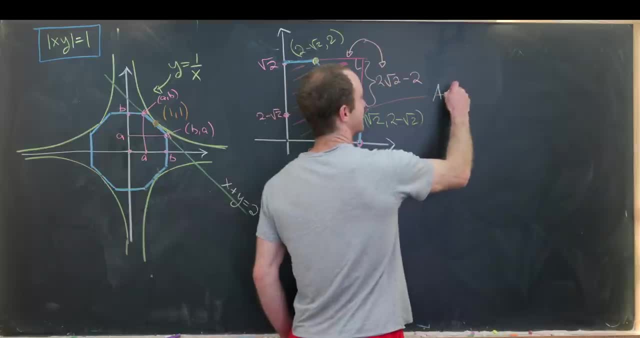 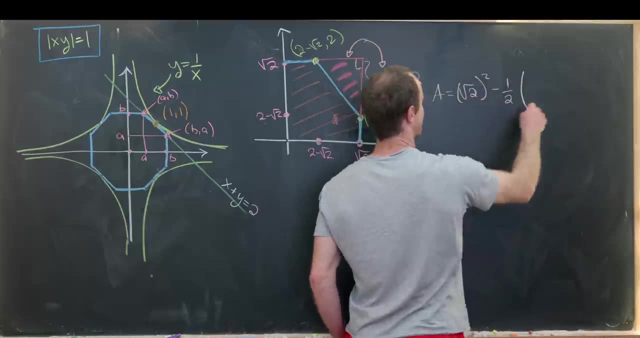 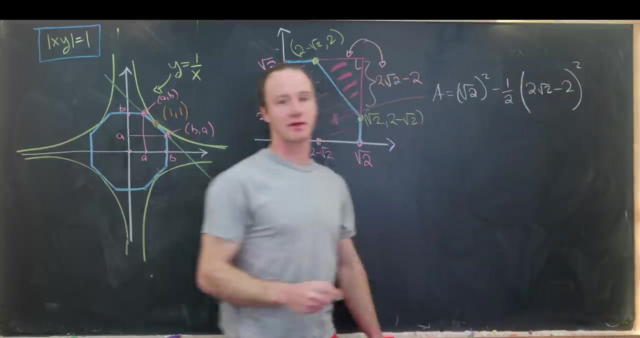 of this brown shaded region is given by the following calculation: So we've got the area of the square. So that's the square root of two squared minus the area of this triangle. But the area of the triangle is two square root of two minus two squared like that. 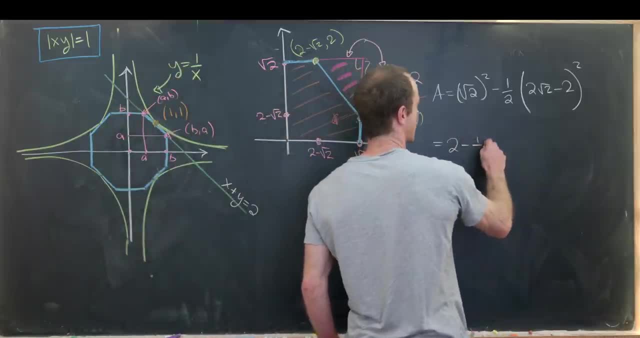 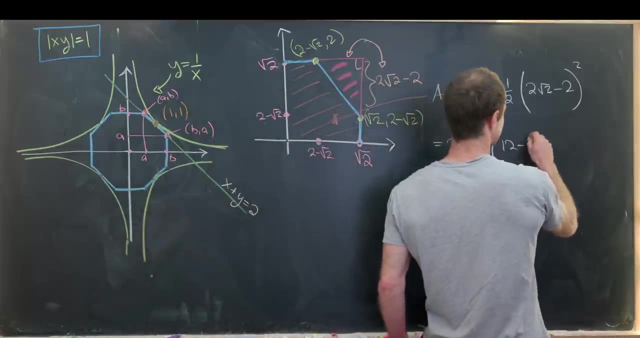 Now let's see what we get. So the square root of two squared is two, and then we have minus 1 1⁄2.. Then, multiplying that out, we'll see that we get 12 minus eight times the square root of two. 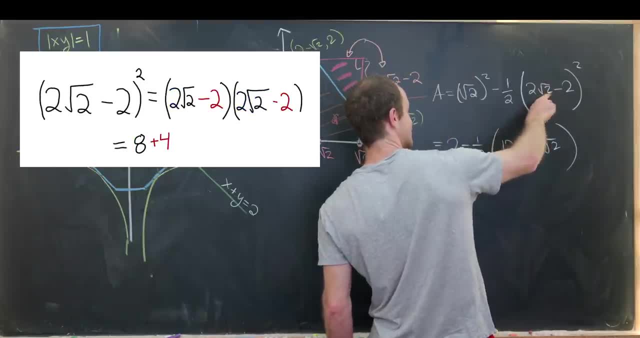 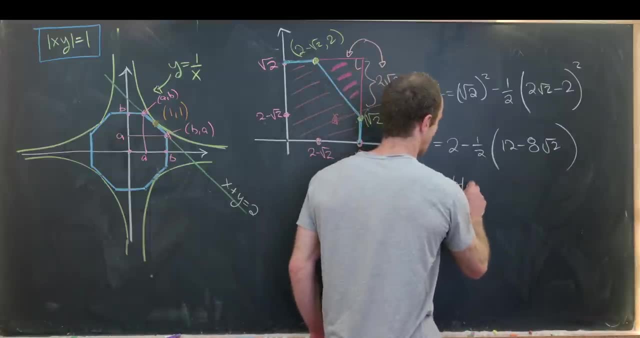 That's because two times the square root of two squares to eight, we have to add four, and then this comes from the cross term. So after doing a bit of simplification, we'll see that this is equal to four times the square root of two minus four. 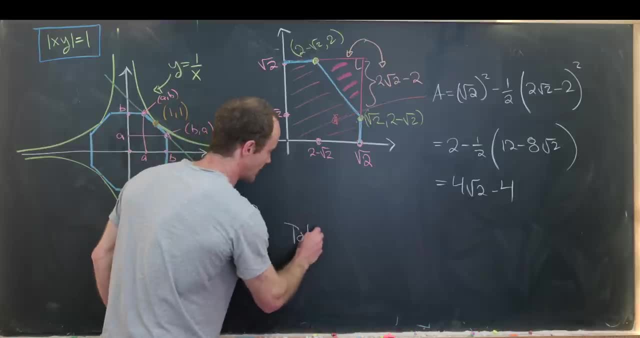 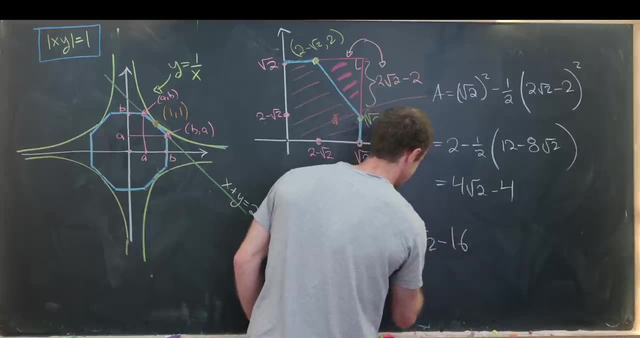 But that's just the area of our brown region. The total area of the octagon that we're looking for is, in fact, 16 times the square root of two minus 16. Which we get just from taking four times this quarter area here. 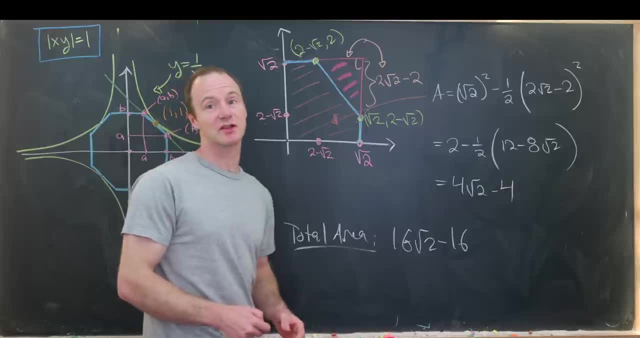 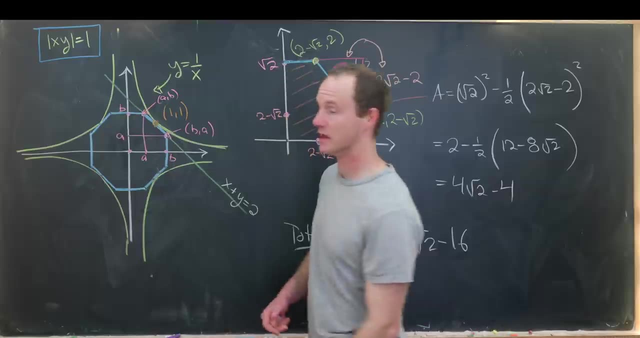 And maybe, before we finish, I'll give you a bit of a challenge question to build off of this. And that would be what happens if we rotate this octagon a bit and we rotate it until one of the vertices intersects- at this point, right here. 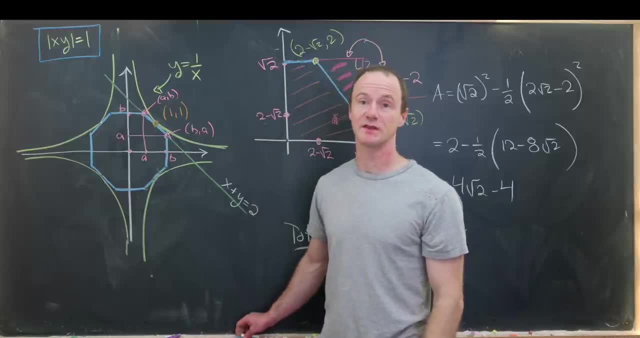 What would the area of that new octagon be? And that's a good place to stop.